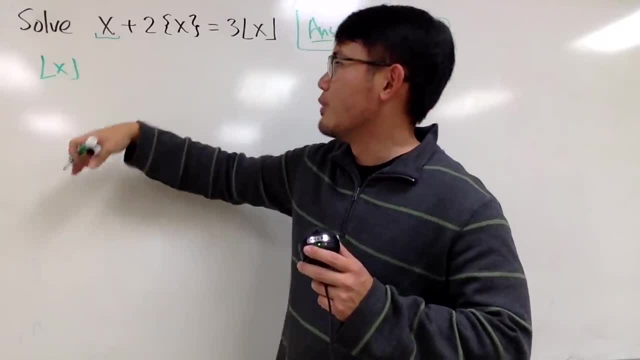 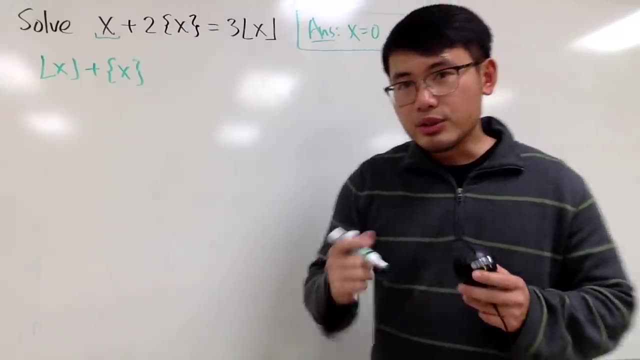 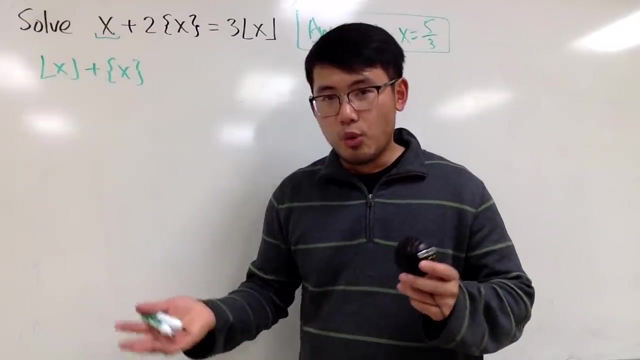 This right here is the same as the greatest integer of x, that's less than or equal to x, right here? or the flow of x, and then we add the fractional part of x. So just a quick example: if x is 4.2, then the flow of x is going to be the flow of 4.2, and that will be 4, and then the fractional part of 4.2 is just 0.2.. 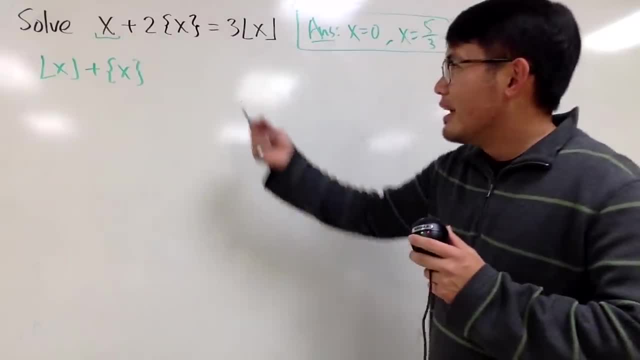 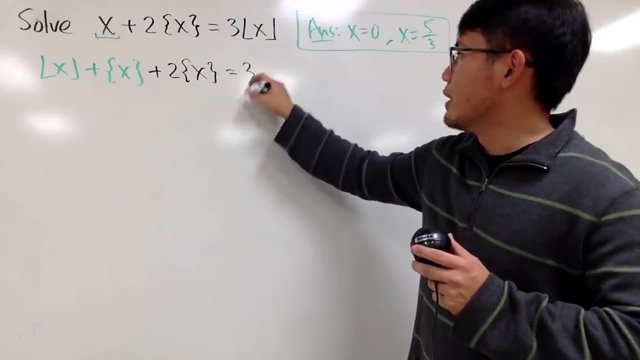 4 plus 0.2,, of course, is 4.2.. So that's the idea, And once you use this right here, you can see that you can combine like terms with others as well. But let me just write down the rest. 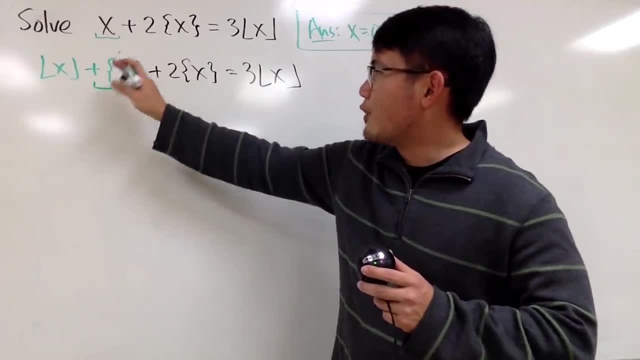 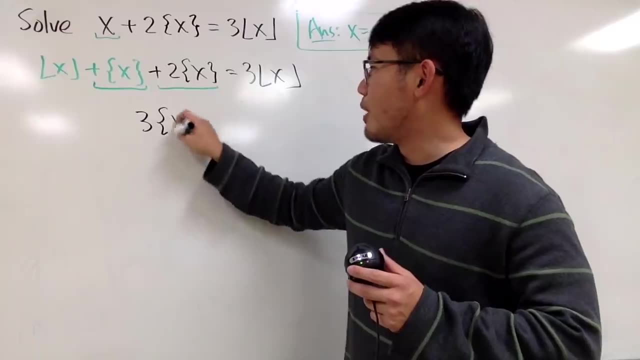 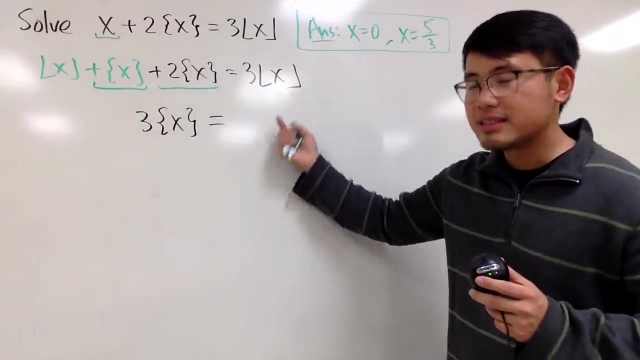 Okay, now we see this right here. we have one fractional part of x and then plus two fractional parts of x. So of course we can just say this is three fractional parts of x, And then I can just subtract the flow of x on both sides. 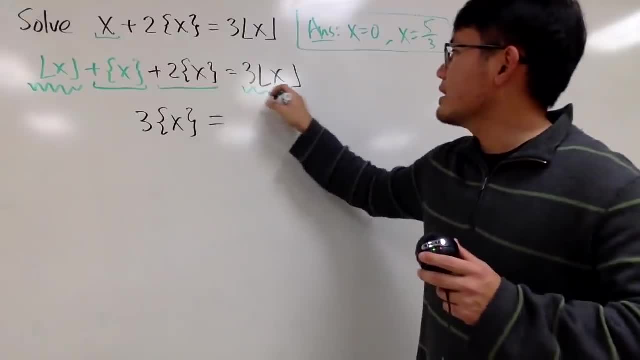 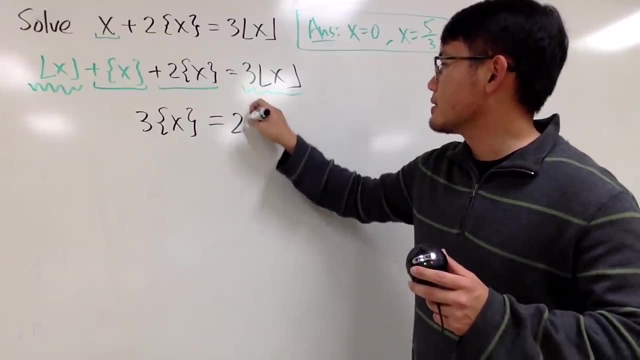 Okay, so you see. Okay, so you see This right here, and that if I bring that to the other side- three flow of x minus flow of x, I end up with two flow of x like this. Okay, now, this is what we're going to do next. 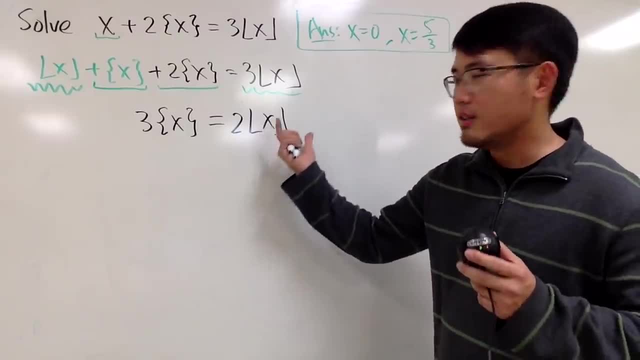 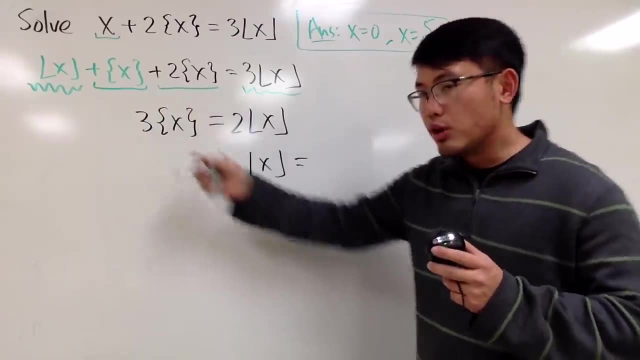 And it depends on how you want to do it. Perhaps I would like to isolate the flow of x. So let me divide both sides by two and we see we have flow of x that's equal to three over two times the fractional part of x. 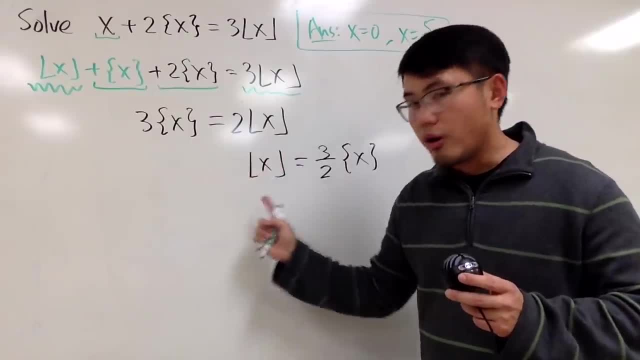 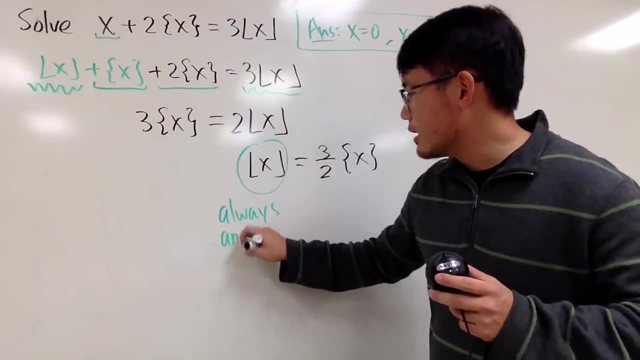 And why do I want to do that? Because remember the flow of x, this right here: it always has to be an integer. So let me just write this down right here for you guys. It's always an integer, positive or negative, whole numbers or maybe even zero. 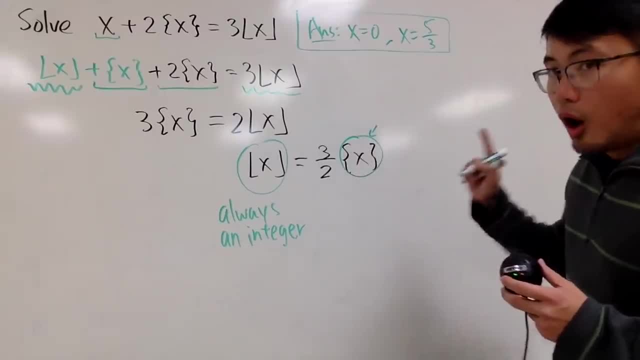 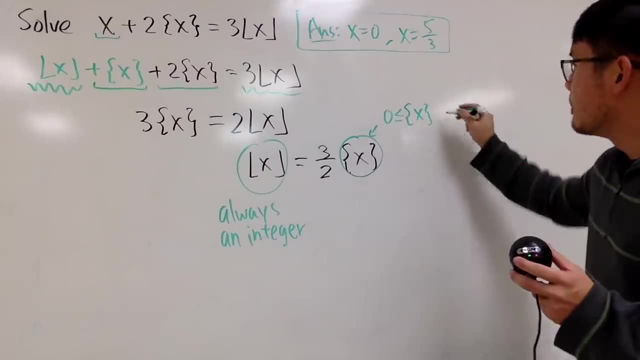 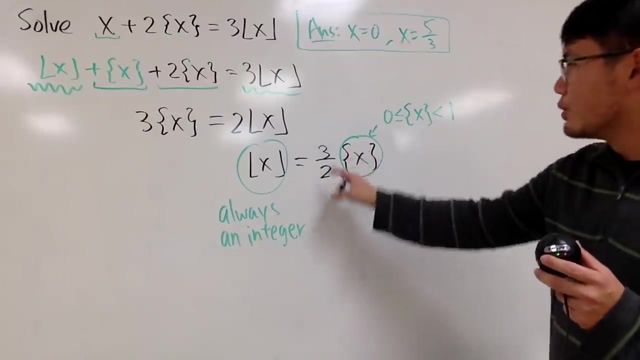 And then, if you look at this right here, we always have the fractional part of x to be in between of zero, and it's okay to be exactly zero, but it has to be strictly less than one. And now you see, here we have an integer that's equal to three over two times, you know, a range from zero to one. 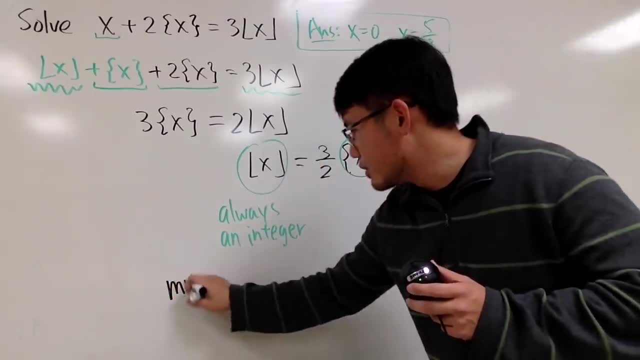 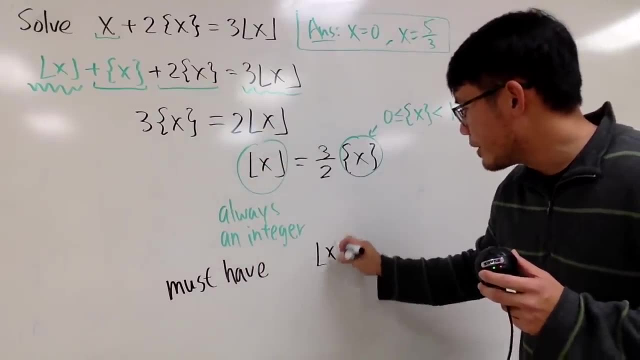 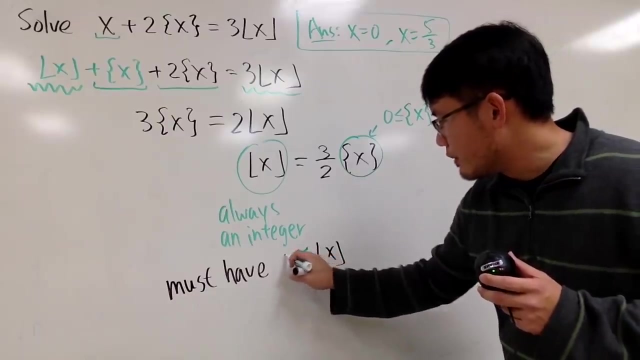 So that means right here we must have- let me just once again write this down: right here we must have the flow of x. right here, You can just imagine: multiply three, half right here and right here. So we end up with the flow of x, that's in between of zero and less than three. 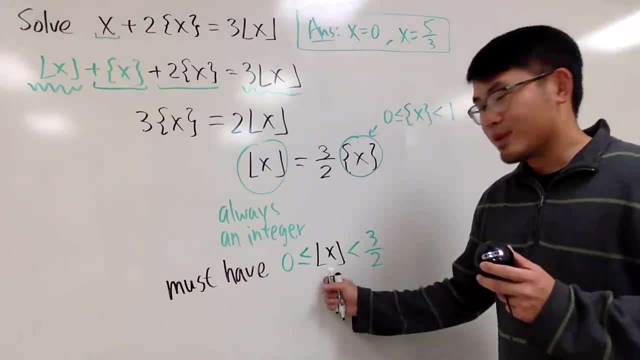 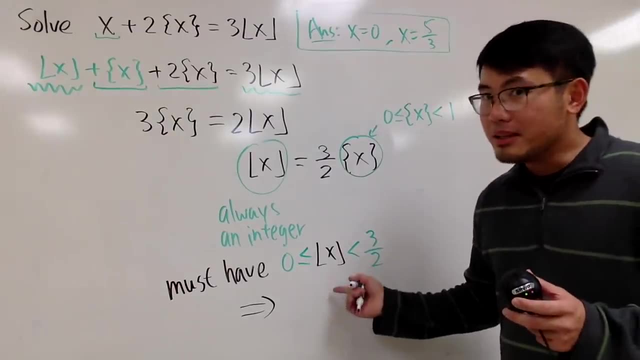 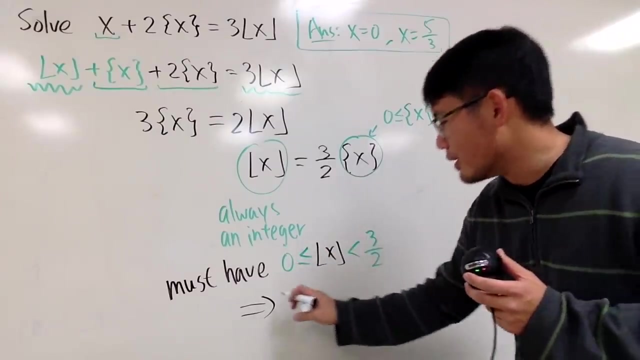 Three half, And now we have this inequality. In fact, we have two situations. So the first one is that, well, give me an integer that's in between of zero, including zero, and less than three half. Well, this right here can be exactly zero. 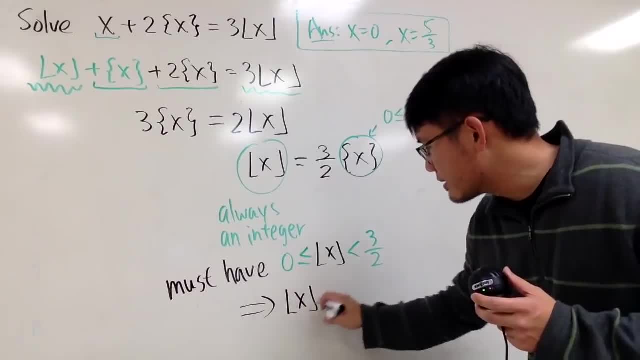 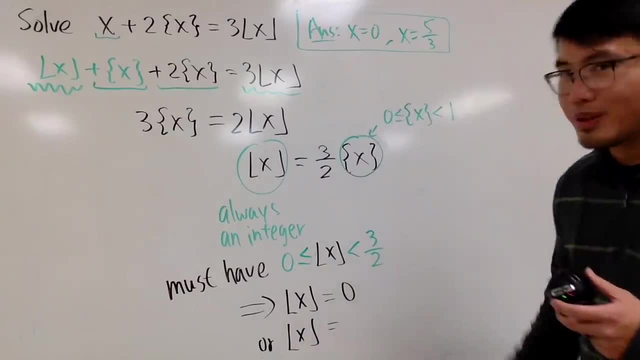 So I will just say: the first situation is: the flow of x is exactly zero, right? Or the second situation is: what's another Non-zero? So this is just an integer that's in between of zero and three half. Of course it's just one right. 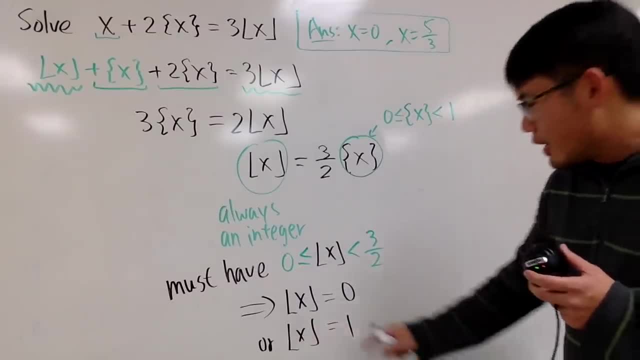 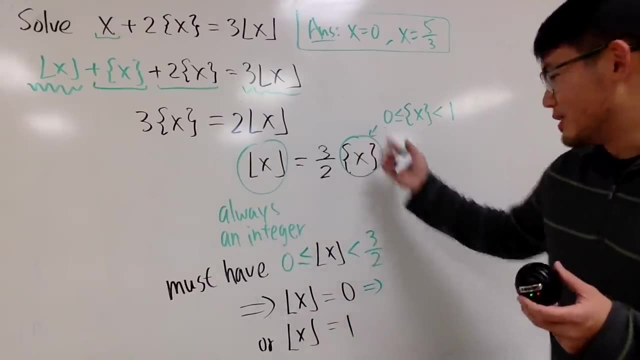 So another situation is: the flow of x is equal to one. From here we know well, if the flow of x is zero, that means this right here has to be zero as well. So that means the fractional part of x is equal to zero. all right. 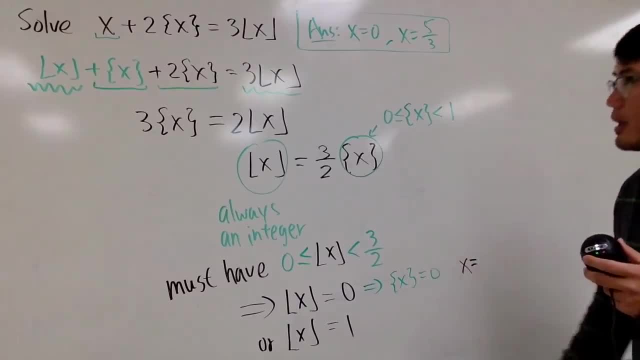 So from here you can say: x is equal to, because we know x is equal to this plus that. so we know x is equal to zero plus zero, pretty much. So let me just write this down right here for you guys: Zero plus zero. 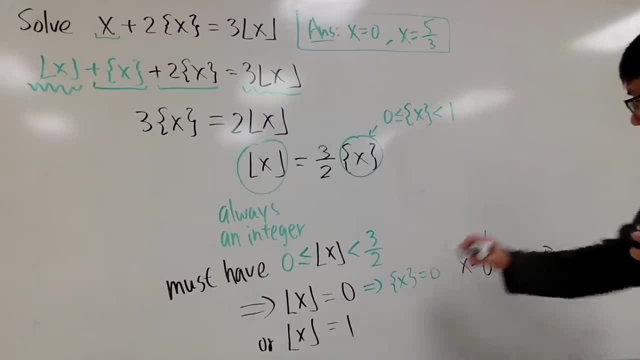 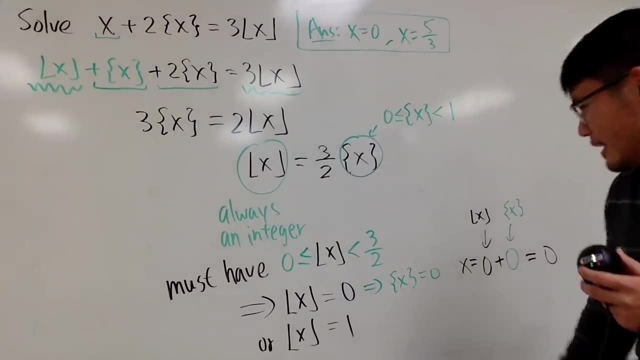 Of course, the answer to this is just zero. This right here is the flow of x, and this right here is the fractional part of x. all right, Okay, from this situation. well, if the flow of x is one, so here we have one. 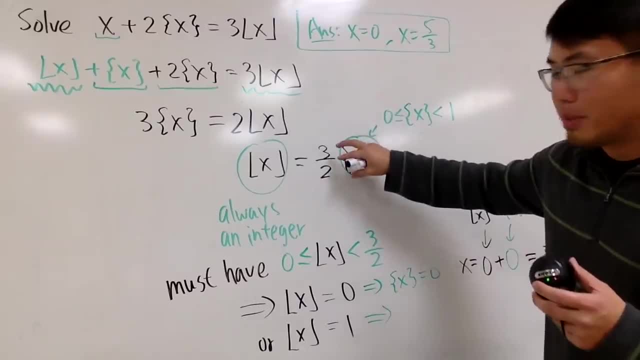 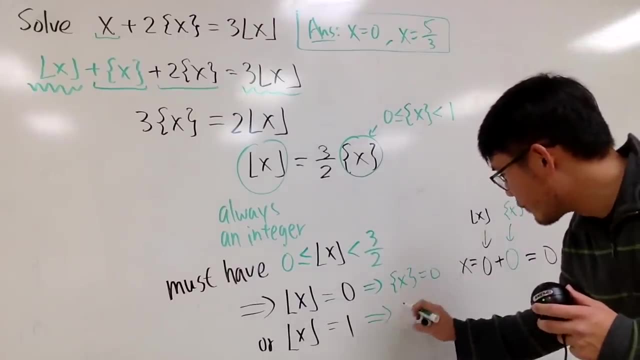 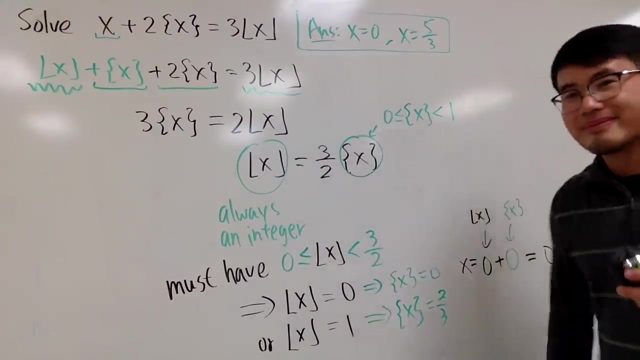 we can just solve for the fractional part of x by multiplying by two over three on both sides, and that is a fraction, right. So you end up with the fractional part of x in this situation to be two over three, If you imagine. if you put two over three right here, of course, you end up with one.